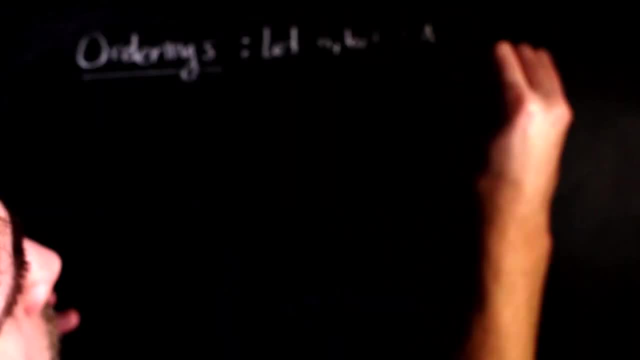 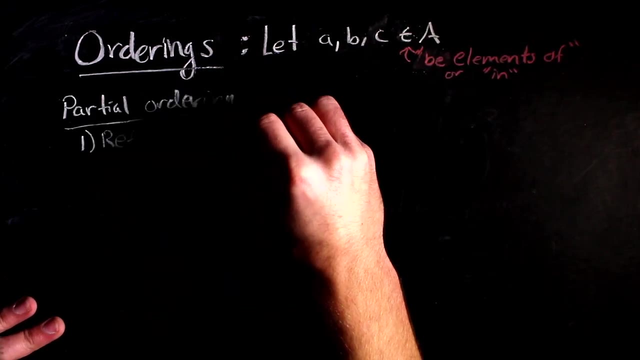 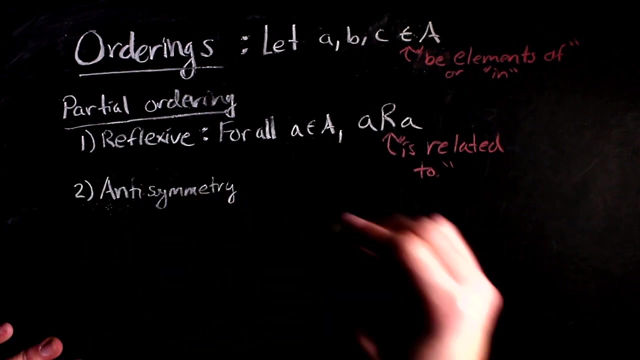 talk about are partial orderings and total orderings. Let's let A, B and C be in our set. A. A partial ordering has three properties. It is: 1. Reflexive, meaning that everything in the set is related to itself. 2. Antisymmetric: if A is related to B and B is related to A, then A equals. 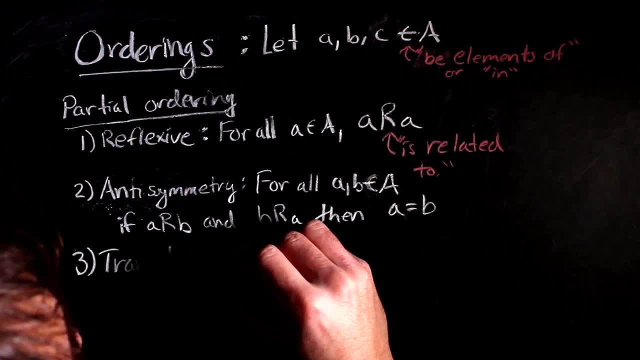 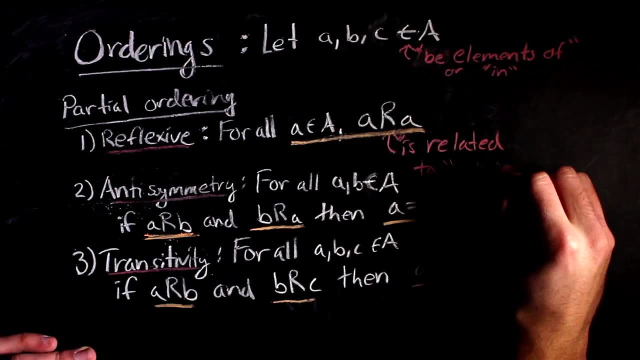 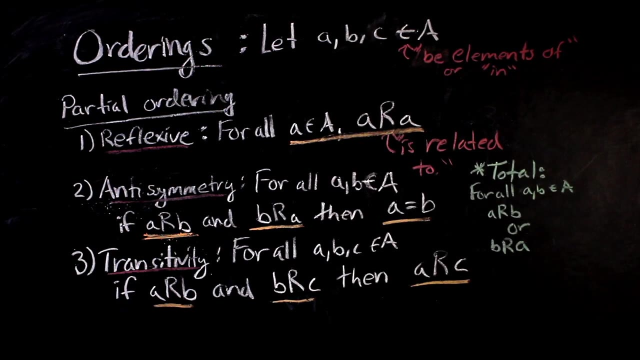 B And lastly 3. It is transitive, that is, if A is related to B and B is related to C, then A is related to C. A partial ordering is called a total ordering if every two elements of the set can be related in some way. Let's look at an example. So if we take the set, 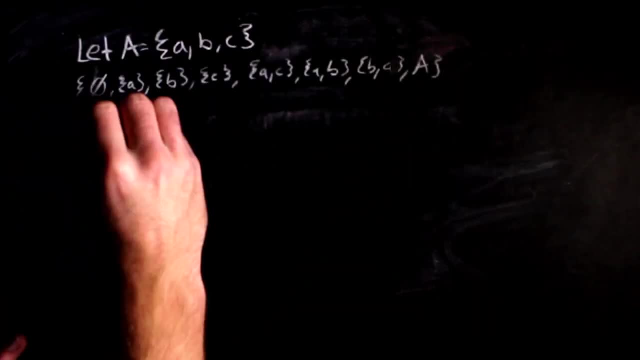 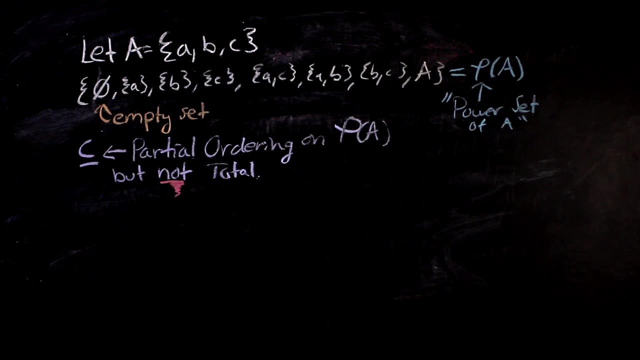 of A, B and C and we take all subsets of that set, also called the power set set. inclusion is a partial ordering but not necessarily a total ordering. This can be proven in general for any power set, but we will show it here for our particular case To show that it's. 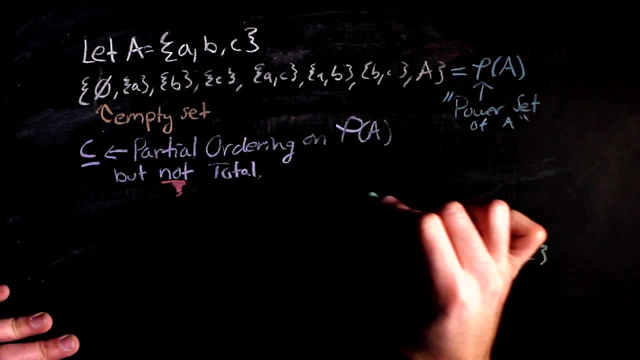 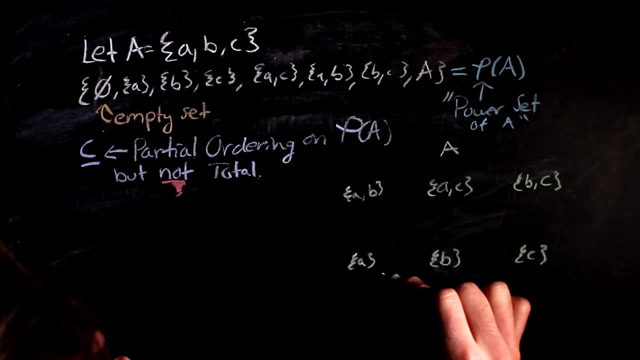 a partial ordering, we can just draw What is called a Haase diagram. A Haase diagram is a directed graph where each element of our set is a vertex and an edge goes from an element x to an element y if x is related. 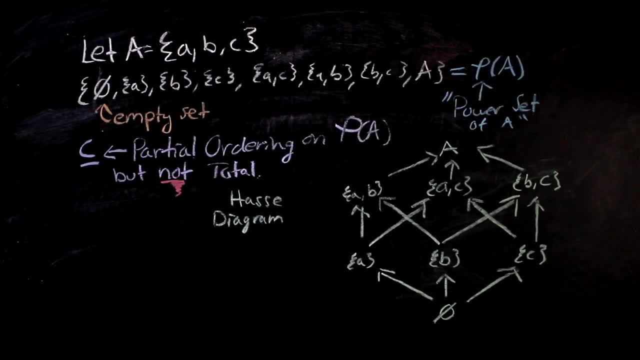 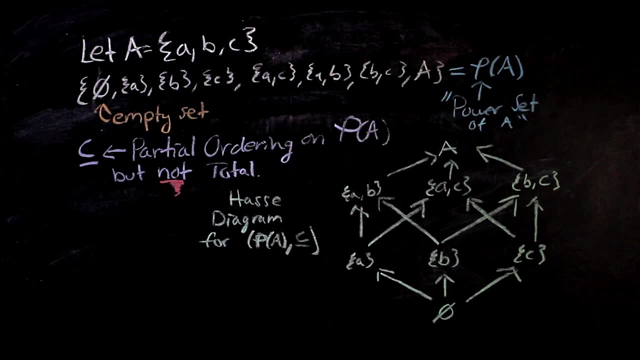 to y And there's nothing z that can be placed between the relation of x and y. Every path that obeys the direction of the edges gives a totally ordered subset of our set known as a chain. So, for example, if we start at the bottom of the Haase diagram, we can see that the 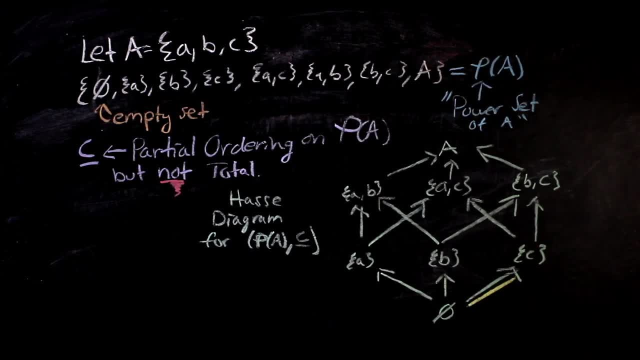 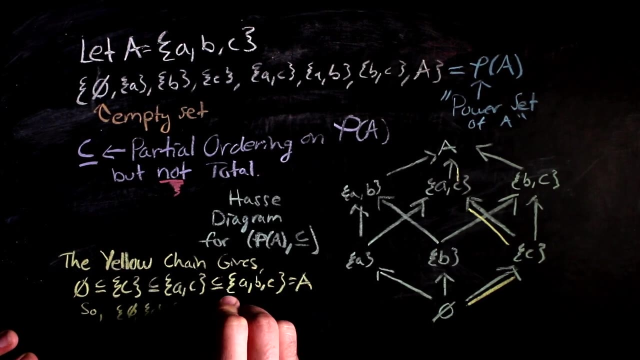 empty set is a subset of the set containing C, which is a subset of the set containing A and C, which is a subset of the entire set A. And so the set of the set A, the set A and C and the set A is a totally ordered subset of the power set, Since there is more. 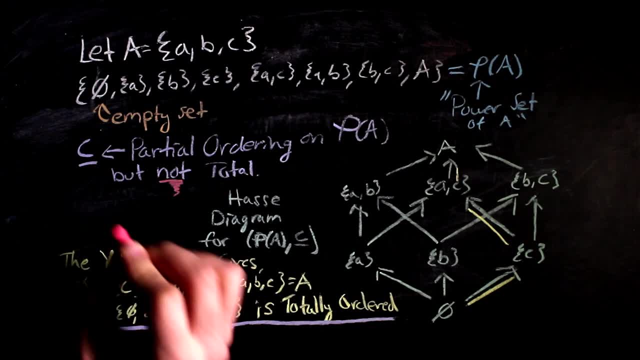 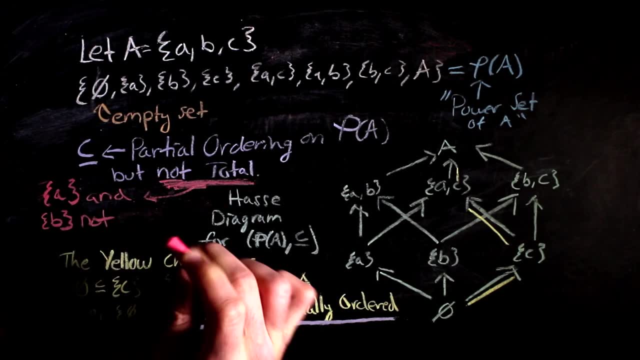 than one chain in the Haase diagram for the power set of A. it follows that not everything is comparable. For instance, the set of A and the power set of A are not comparable. For instance, the set of A and the set of B are not comparable as there is no chain that contains both of. 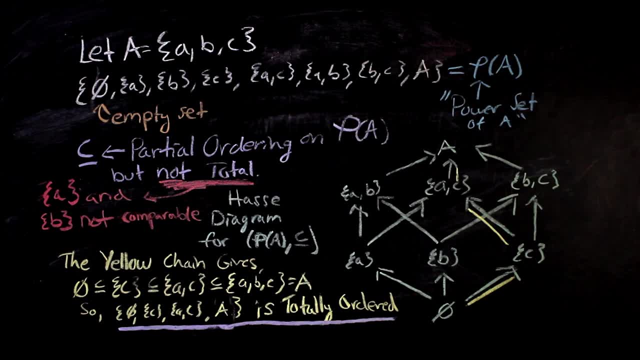 them. So the relation is not a total ordering. It is a short exercise to see that the transitive, anti-symmetric and reflexive properties are all presented by the Haase diagram as well. If you're not convinced, now would be a good time to stop and think about it before continuing. 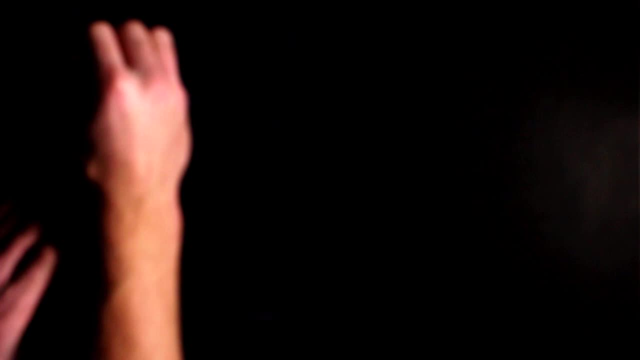 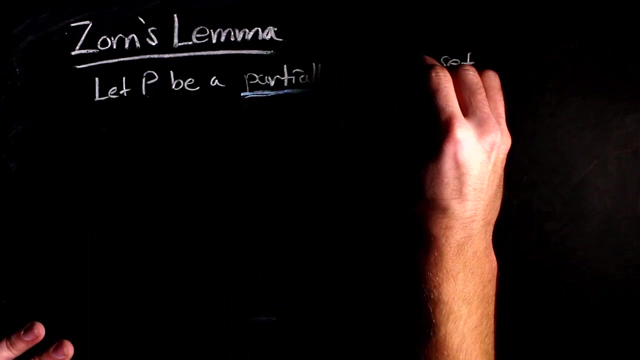 on. Now that we're a bit comfortable with orderings, we can begin to talk about Zorn's Lemma, which can be stated as follows: Let P be a partially ordered set, such that every chain in P has a P. Then the set P contains one maximal element. Here, maximal just means that there 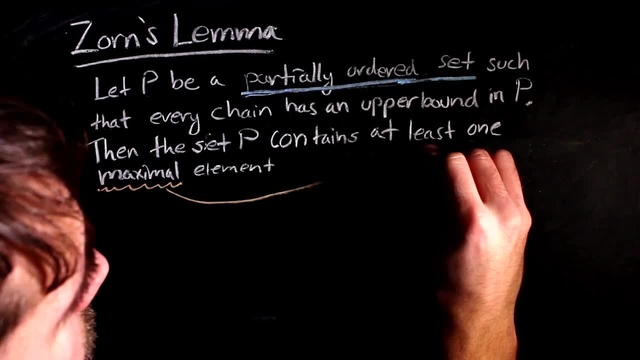 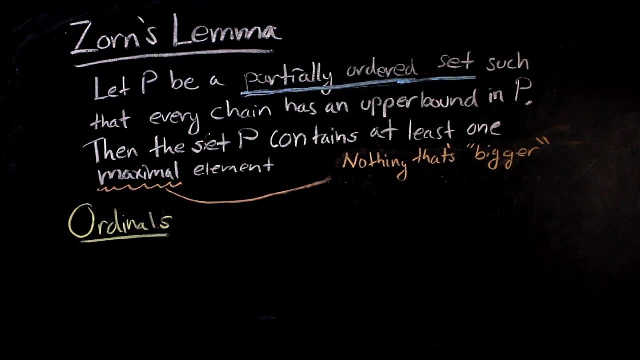 is nothing larger in the sense of the ordering imposed on P. Before we continue with the sketch of the proof, there is one tool that is required: The ordinals. The ordinals are generalization of the natural numbers. So we have 1,, 2, and. 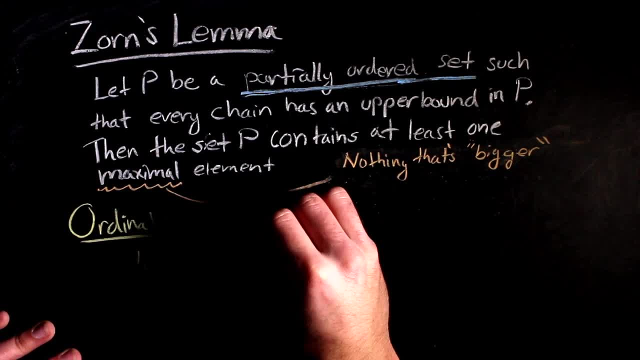 3, all the way up to omega, which is the symbol that denotes the size of the natural numbers. After omega, we just continue counting as usual: Omega plus 1.. I'll say that I'm just going to go ahead and count down to 1.. If you've any questions, just let me know. I'll talk to you later. 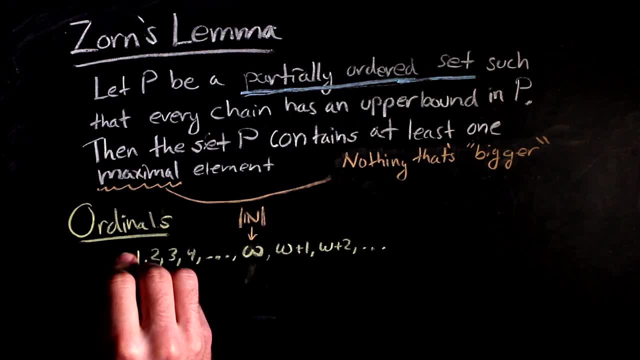 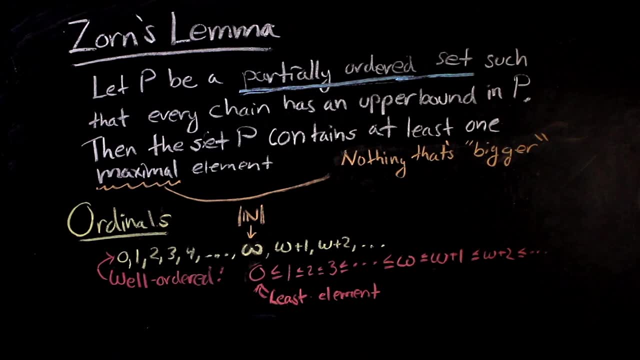 omega plus two, omega plus three and so forth. First, this collection is well-ordered, which just means that there is a least element for every collection of ordinals, And, second, that there are more ordinals than there can be elements in any set, because, 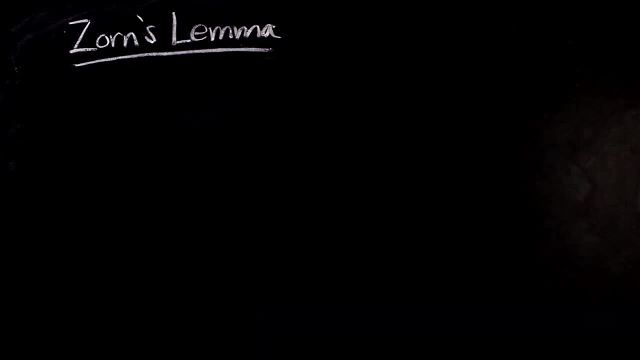 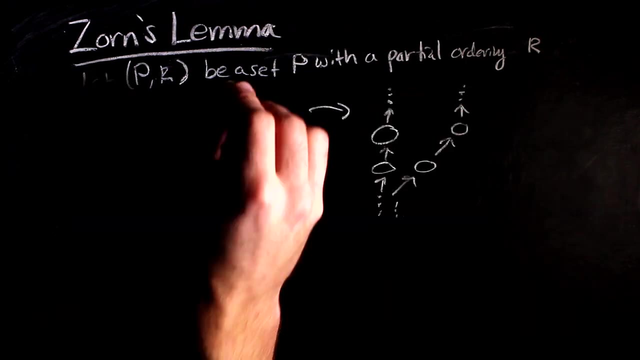 there is an ordinal for every possible size of a set. These two facts about ordinals allow us to show Zorn's lemma by contradiction using Hasse diagrams. Suppose that P is a partially-ordered set, such that each chain has an upper bound and 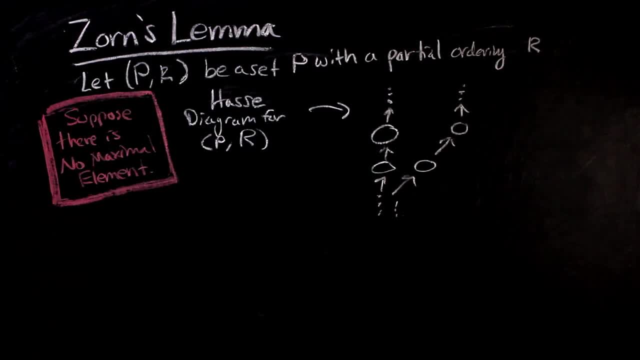 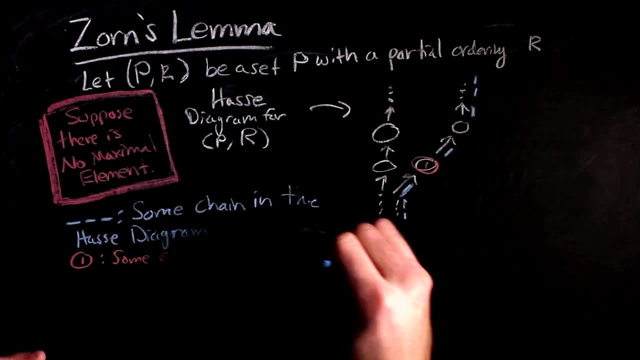 suppose that there is no maximal element For each chain. we can find an element and then choose an element that is bigger because there is no maximal element. However, this is where we encounter a problem. We should be able to go on finding bigger and bigger elements forever, and these elements. 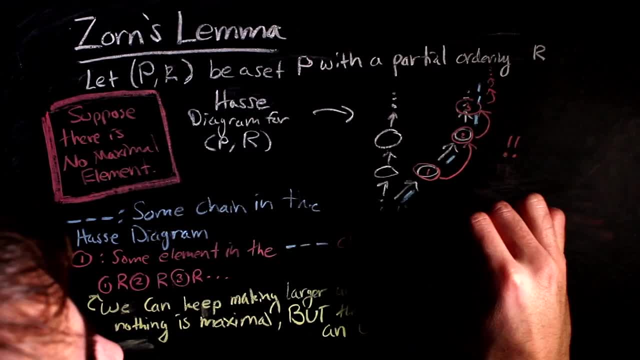 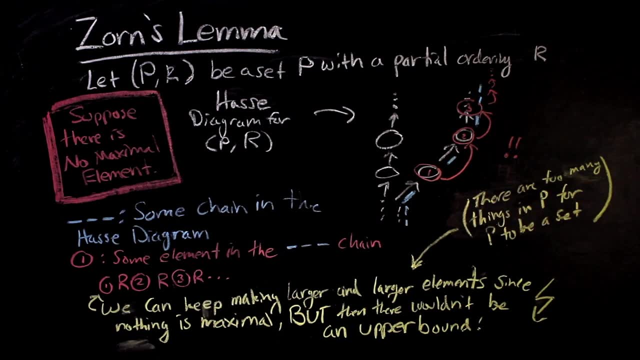 are ordered so that they're the same number of them as there are ordinals. In other words, since there are more ordinals than there are elements of a set. In other words, our set P cannot possibly be a set. it's just too big and that's. 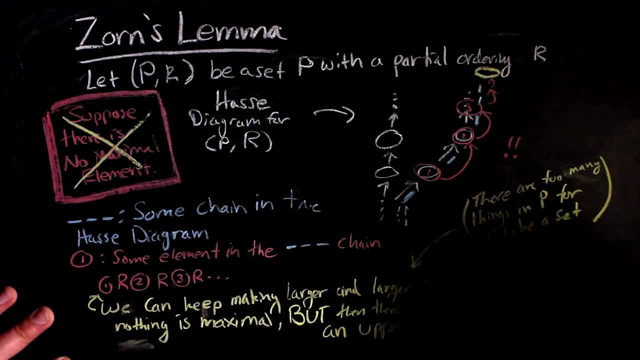 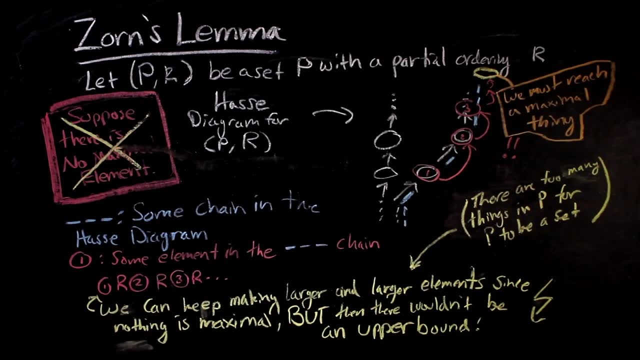 a contradiction. Therefore, we will reach a point where there is not something larger in P and, by definition, we will have a maximal element. Therefore, Zorn's lemma holds by contradiction. The proof we went through, or sketch of a proof that we just went through, used a lot. 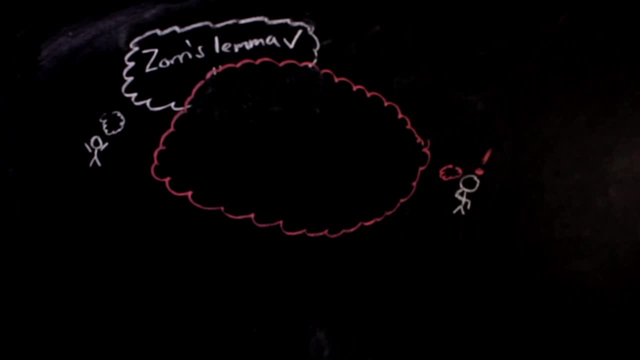 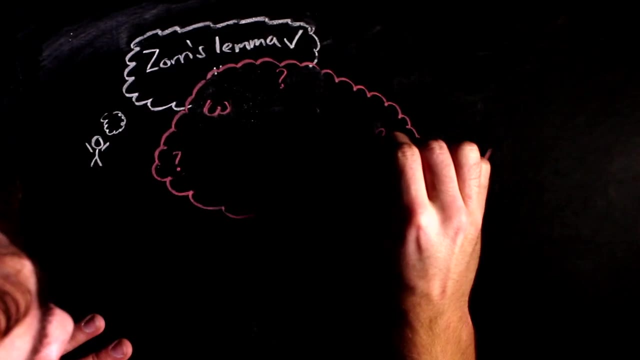 of different weird technical mathematical notions from set theory, the ordinals probably being the most mind-bending. but it also used choice, which is an axiom that can cause quite the stir in intuition. However, the mental stretch of Zorn's lemma doesn't end here. 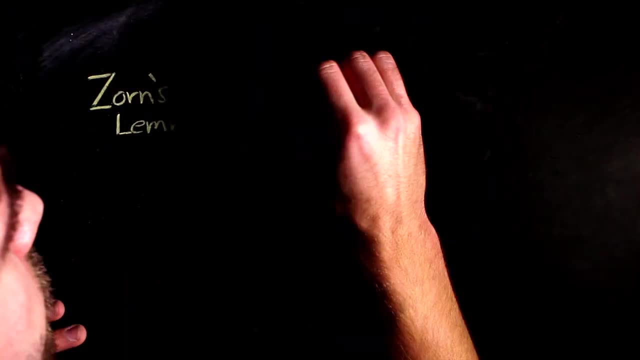 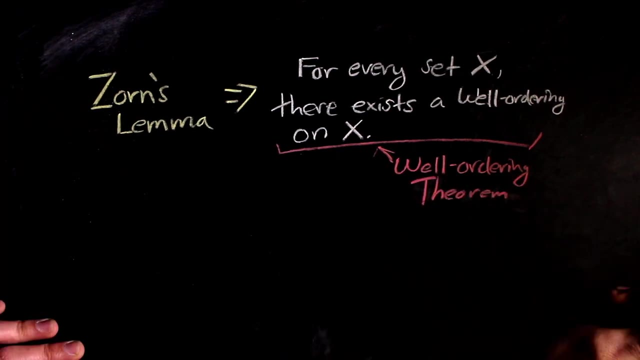 Zorn's lemma can be used to show the following theorem: For every set X, there exists a well-ordering on X. This is otherwise known as the well-ordering theorem. It seems like a simple statement, but it's incredibly hard to think about. for sets with, 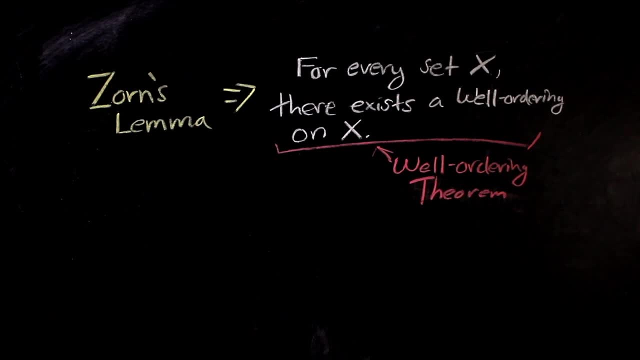 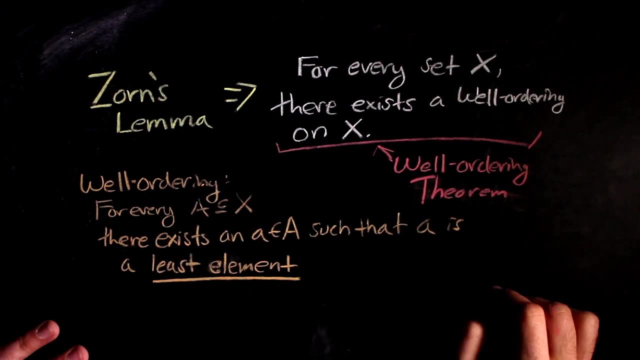 lots of stuff in them. Remember that a well-ordering means that every subset of your set X has a least element. So what happens with the real numbers? We have a notion of a total ordering on the real numbers less than or equal to but this: 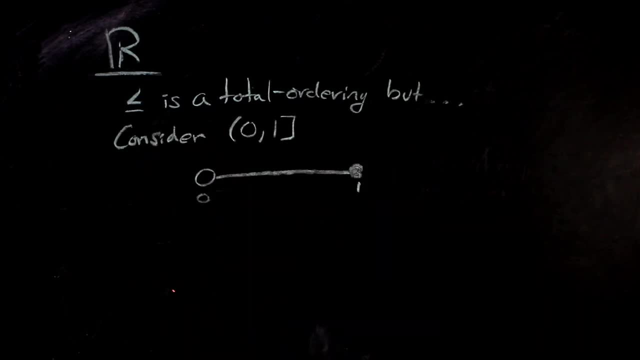 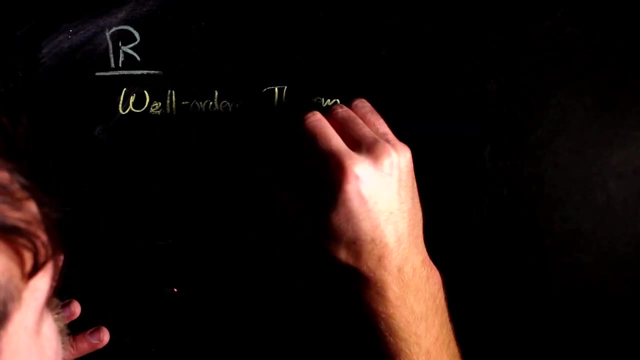 ordering is not a well-ordering because open intervals would not have least elements. In fact, even though this theorem grants the existence of a well-ordering on the real numbers, it has been shown that this ordering cannot be defined in a set-theoretic sense. 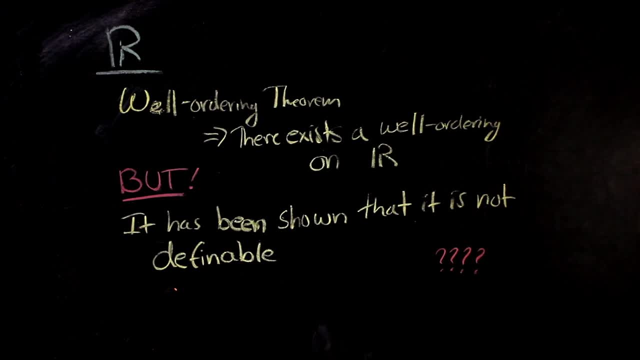 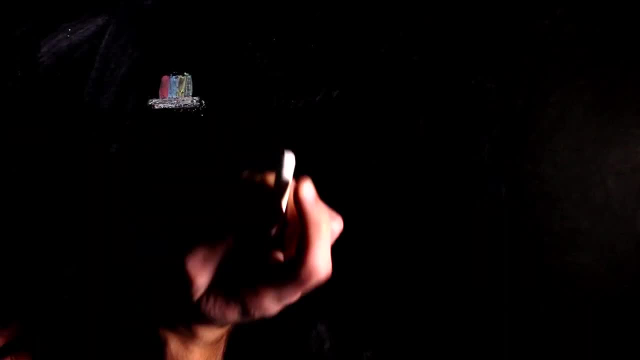 A bit unsatisfying, but that's really all we have for this video. I know I've been gone for a while and I'll kind of not be around that much. I'll see you next time. Thank you so much for watching and I'll see you next time.